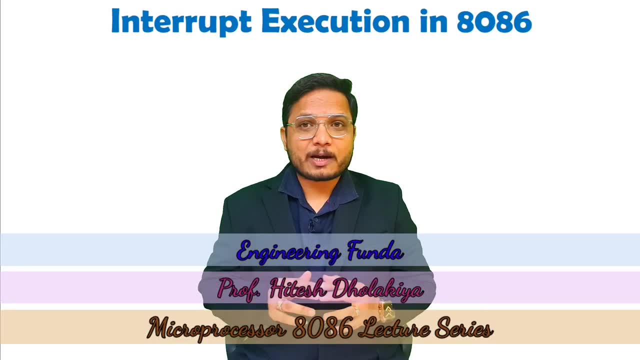 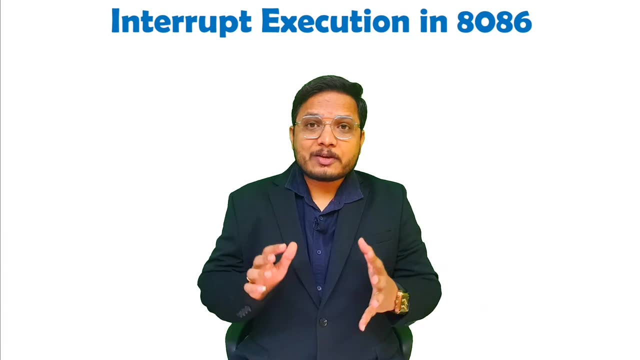 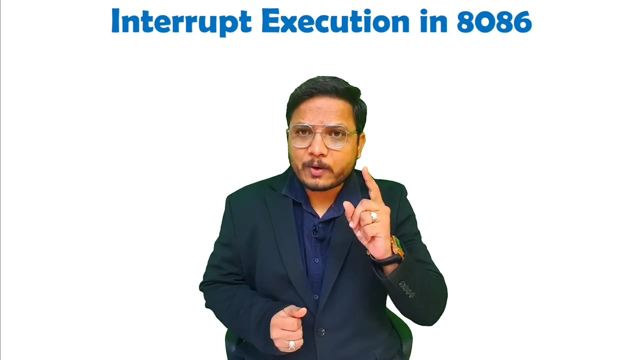 Welcome to Engineering Funda family. This video is a part of microprocessor 8086 video lecture series And in this video I'll be going to explain you execution of interrupt in 8086.. So each and every steps of execution of interrupt that I'll be going to explain you step by step. 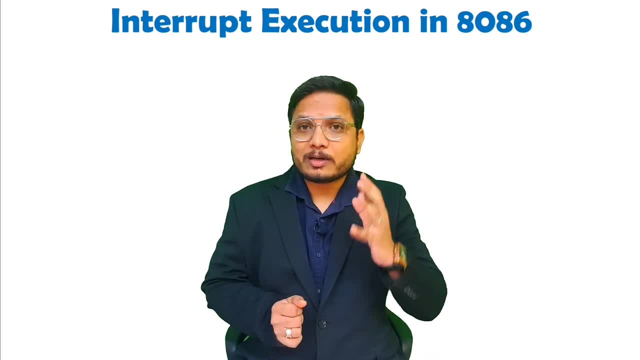 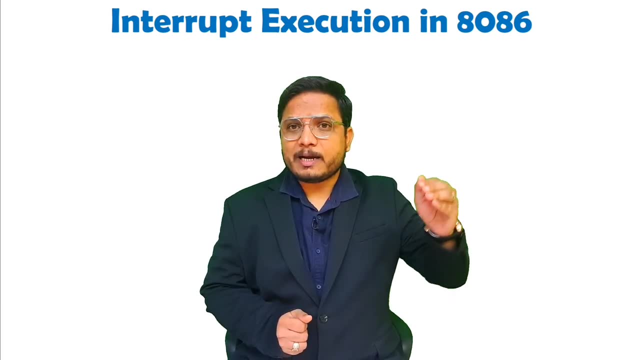 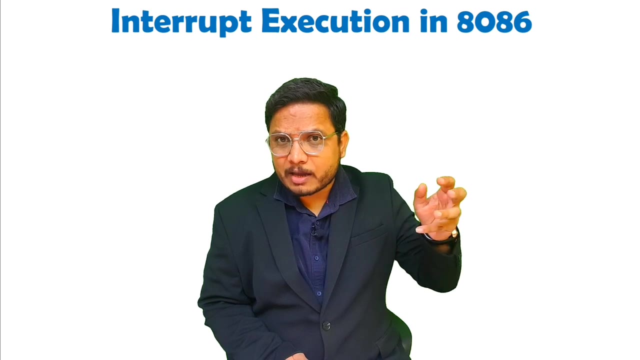 So what I want is you should see this video till last to understand what is the exact process of execution of interrupt with 8086.. Here, my dear students, when you execute main program, and while you're executing main program, in between program, if interrupt comes, 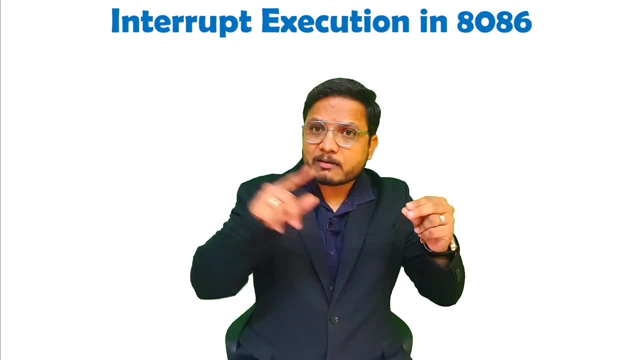 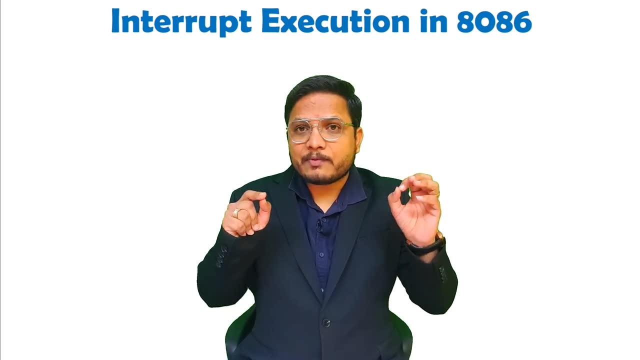 then 8086 will have to give service to this interrupt, And how that service will be given to this interrupt. for that there are a few basic steps that you should know. So let us see it step by step. So, my dear students here, 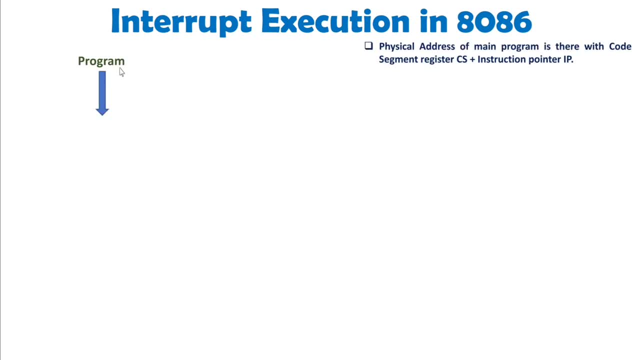 let us say we are having main program that we executed over here, And here with main program there are a few basic things that you should know. Main program is having physical address and that is there with code, segment register CS and instruction pointer IP. 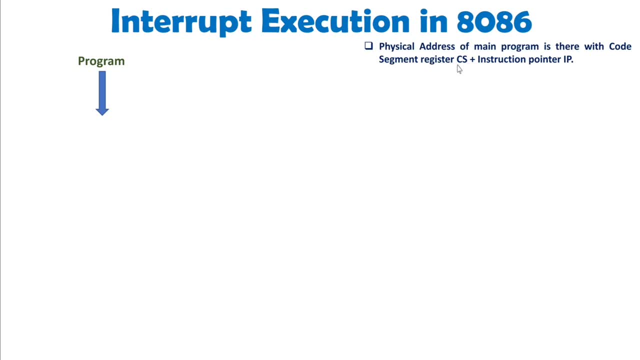 This main program's address is there as per CS into 10 hex plus instruction pointer. So you can say higher address of main program is there with CS and lower address of main program that is there with IP. This IP is offset pointer and this code segment register. that indicates you. 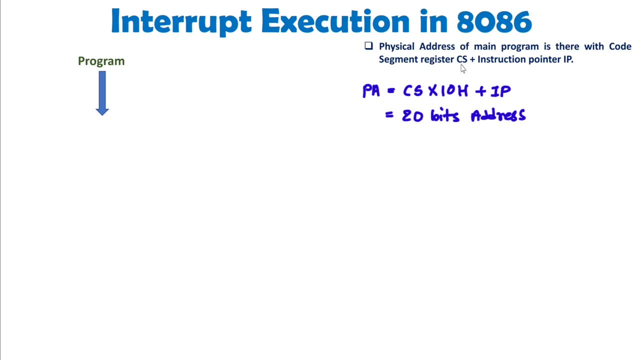 what will be starting address of code segment? right? So you can say: higher address of this main program that is there with code segment register and lower address that is there with instruction pointer. Now when you execute program step by step, one by one instruction, let us say: interrupt comes. 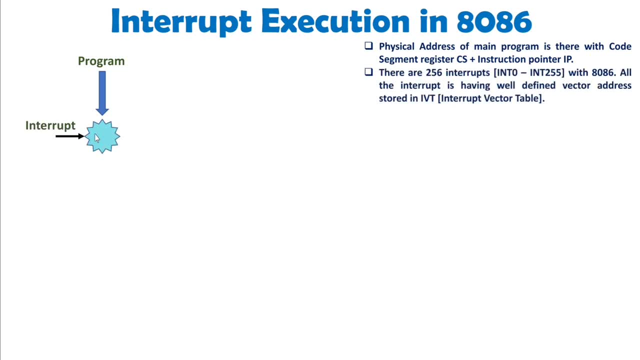 over here. Now you'll be observing, with 8086, there are various interrupts. There are total 256 interrupts, int 0 to int 255.. And all these interrupts are having well-defined vector address And that vector address is stored in interrupt vector table. 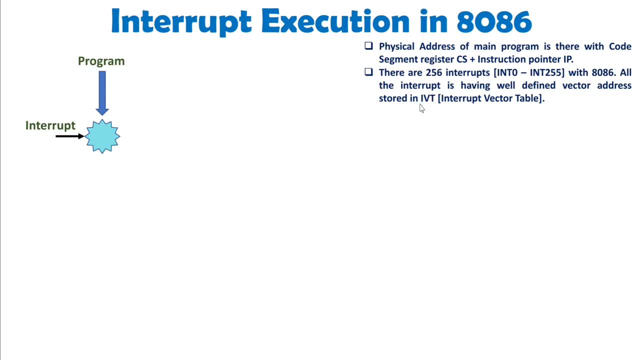 For interrupt vector table. I'll make one separate video Here right now. just consider all the interrupt is having well-defined memory location and that is stored in interrupt vector table, right? So what 8086 will have to do? 8086 will have to take address from this IVT and at that address. 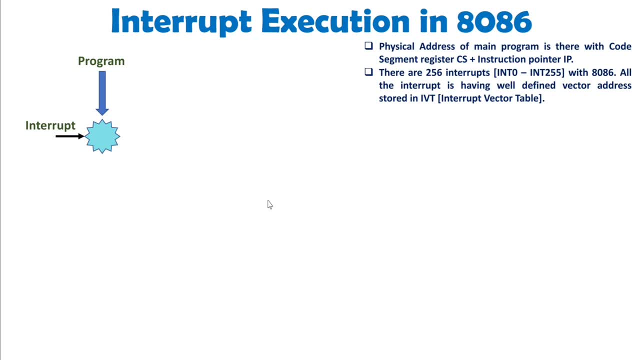 whatever program is there that 8086 will have to execute. But it is not that simple, my dear students Here. there are few more basic things that we need to see Here. we are executing main program During main program, as if interrupt comes then. first of all, 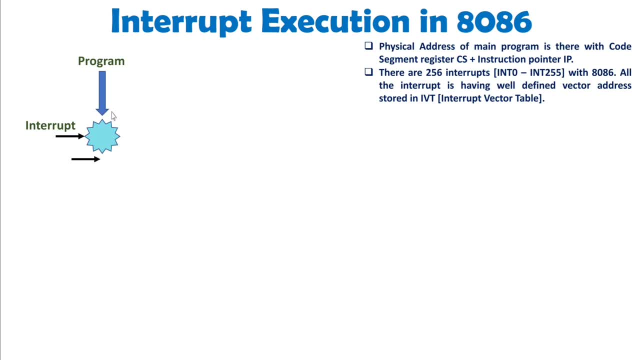 8086 will have to execute current instruction. So, once it executes current instructions, there are few basic things that you should know. First is what is status of this program? So status of this program that will be there in flag resistor, and second is what will be next address of instruction, so next address of. 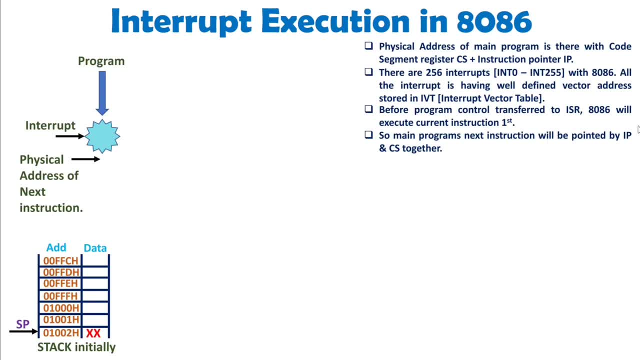 instruction that will be over here and that will be there with ip and cs. right now. higher address will be there with cs and lower address is there with ip. that you will have to consider right, as code segment holds higher address and ip holds lower address. now here with main program status. 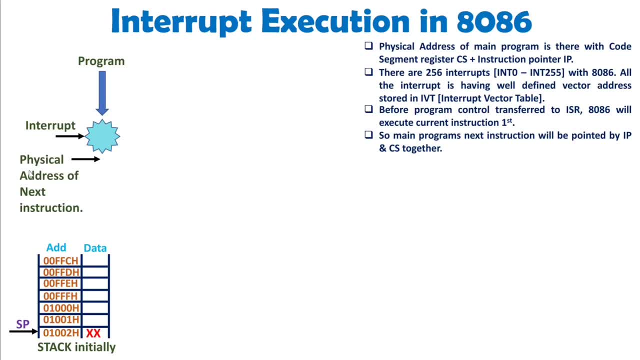 of program and physical address of this next instruction that we need to store on stack. why we need to store it on stack? the reason is, once you complete interrupt service is you will have to come at this physical address along with same storage which is the main plate of this instruction. so podéis come at this physical. 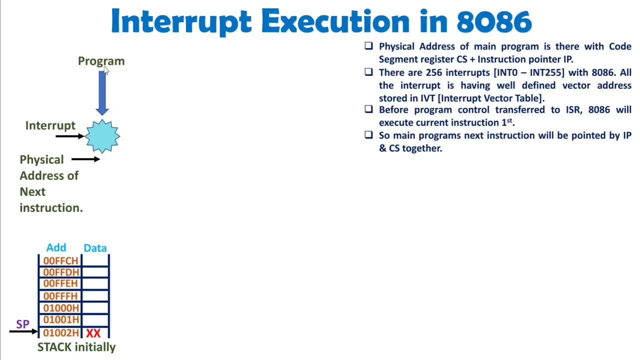 address, along with which same storage, which is the main plate of this instruction. so in this example- status of flag- The reason is you don't need to erase your main program. You need to execute main program as it was there. Only thing is, once interrupt comes, you'll have to give. 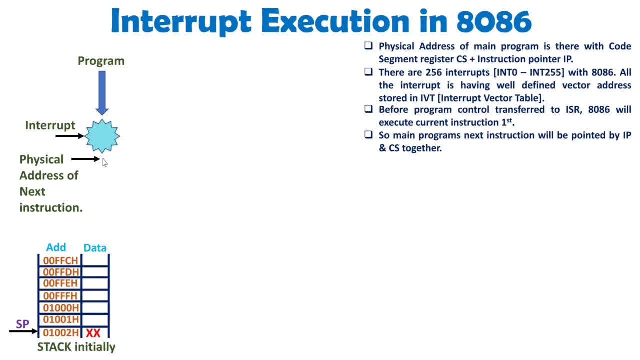 service to this interrupt. Once service is completed, you execute main program, right. So here we need to store status of program means flag on stack, as well as we need to load this physical address on stack. You see how we do that. So first of all, what we do. 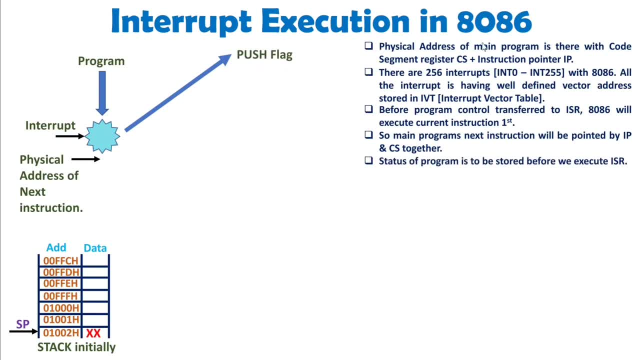 is we perform push flag. So here 8086 is doing this operation, right, We as a programmer, we are not writing this instruction. 8086 will execute push flag first. So what it does, It will be loading status of flag on stack first. After that, what it does is it will: 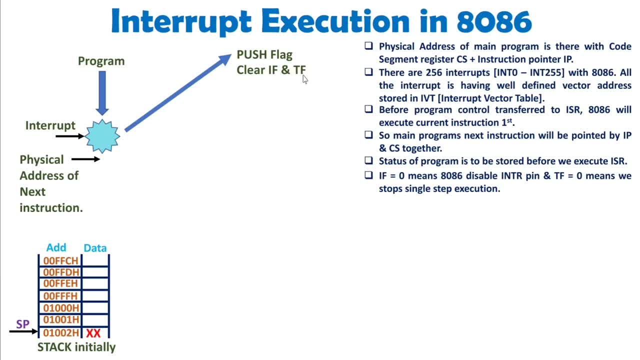 clear 8086. Interrupt flag and trap flag. Why it clears interrupt flag and trap flags, My dear students, when it clears IF it will be doing disable INTR, pin What it means Now. INTR cannot give interrupt to 8086 as already this interrupt is there under service and trap flag will be. 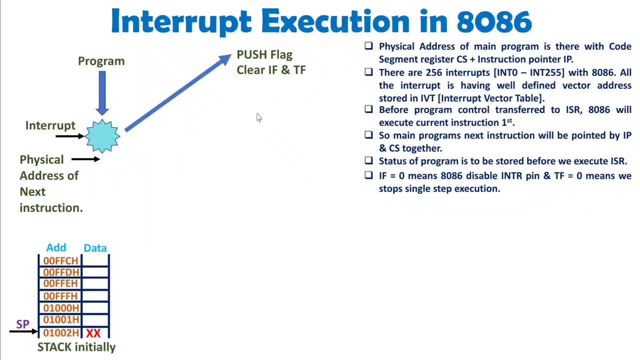 cleared over here Why The reason is here. service to interrupt cannot be done If the ITERP will not be shoot a drop flag as per single step, right. So you will have to execute this service to interrupt in a one go. You don't need to do this as per step. 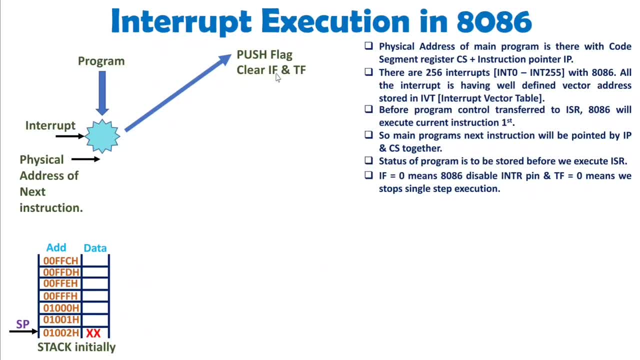 by step. So first of all, 8086 will clear if and tf. After that this physical address of next address with this main program that will be loaded on Stack. So here you see, first we are doing push CS and then we will Grid pregunta right Counter. sketching function efficiently. you see its working Alright. soogn dellaفس is an activity which makes, obviously when we have added the values it will, suggestinations of, such as my entrepreneurship to other plans. So here you see. first we are doing push CS. 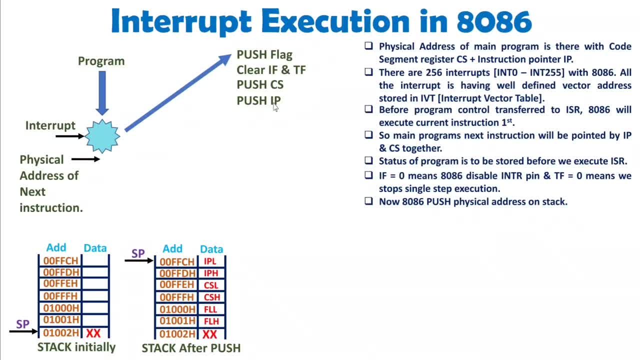 Thank you very much. Thank you very much. do push ip. so here what we do is we load physical address on stack. you see, here we have loaded physical address on stack. now you might be having question why we have loaded this code segment register first. after that we have loaded ip on this stack. so why this sequence? 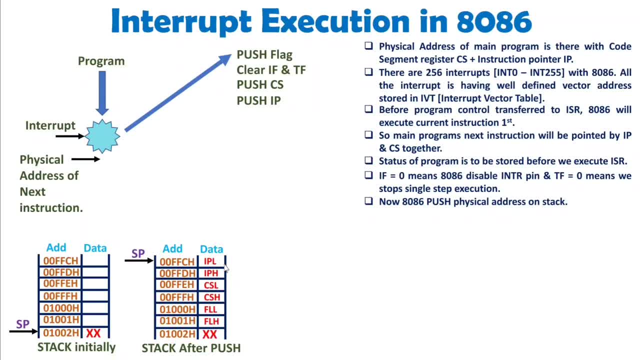 is there. so you should know, my dear students, with 8086 or with any intel processor, we are loading physical address as per: lower address at lower byte and higher address at higher byte. so what i have explained here, you see, i have told you segment register that holds. 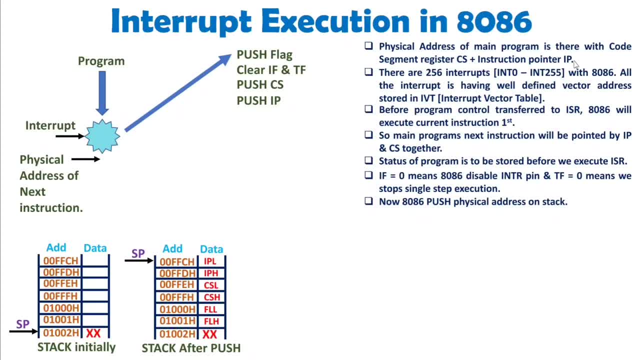 higher address, higher address and instruction pointer that holds lower address. so lower address that we load at lower value of address location and higher address that we holds at higher value of address location of stack. so you see, when you do push operation, address will get decremented and here cs will. 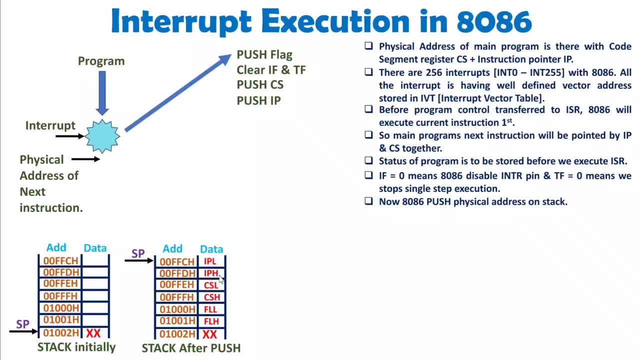 be loaded first as it holds higher address, and after that ip will be loaded at. lower. IP will be loaded as it holds lower address, right? thats why sequence is like this: right now, once you have loaded this flag and physical address of main program, all you need to do- 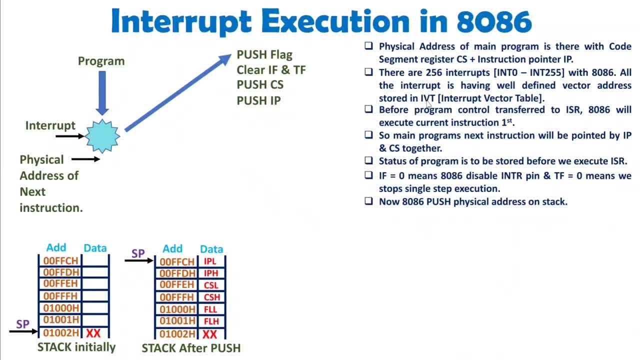 is. you need to see inter beaucoup table. So 8086 will load physical address of program from interrupt vector table. how it will be loading address. so it will be taking it from interrupt vector table. so isr interrupt service routine that will be taken from interrupt vector table. for that i'll make separate video and in that i'll 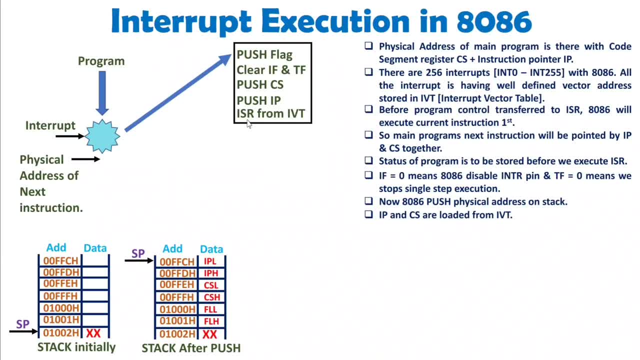 explain you how it will take physical address right now. consider for isr 8086 will take physical address from interrupt vector table. so ipncs now loaded from interrupt vector table, so now you can execute interrupt program. so here we are, executing interrupt program and at last. 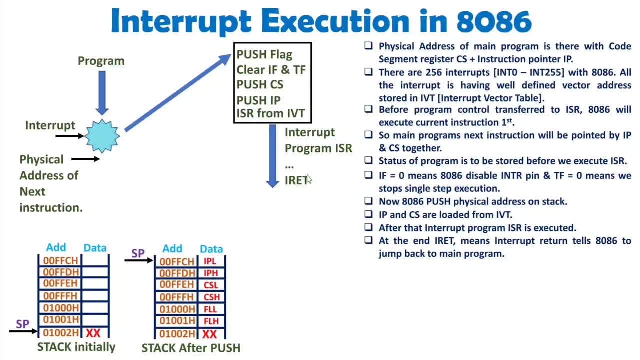 i return is executed, which indicates interrupt service is completed. see, it is not ret, it is i r. e. t means interrupt return. there is a difference between normal return and interrupt return. that even i'll explain you once i complete this. once you execute, i return 8086 will have to. 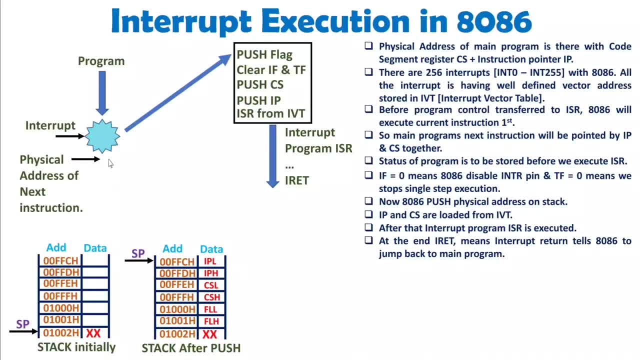 jump back to the previous video and i'll explain you how to execute. i return 8086 will have to main program, but it cannot directly jump to main program. it will have to take this address as well as it will have to take status of flag, right. so what it does is it will be doing pop ip, pop cs and 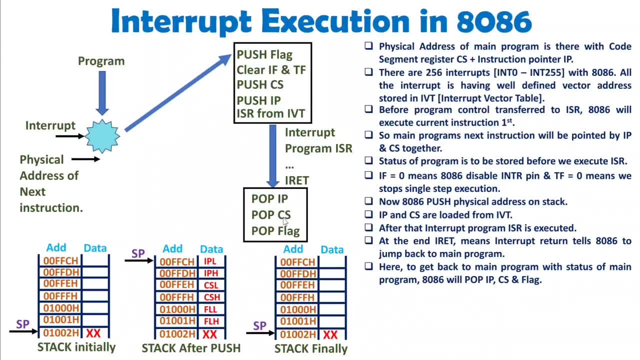 pop flag, why it executes it in this sequence. the reason is now, you see, stack is operated as per last in first out. so now you will have to do pop ip first, after that you'll have to do pop cs. after that you'll have to do pop flag as per last in first out, right? so this sequence will be there. 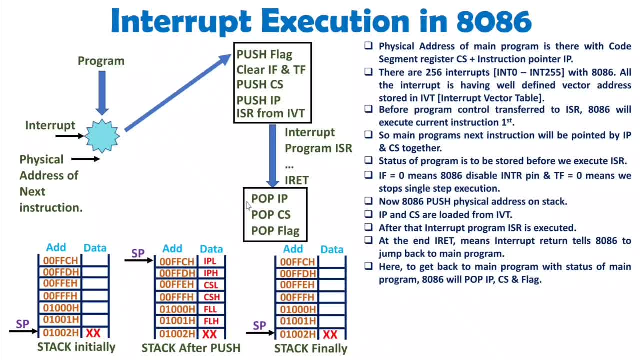 and once it does, this pop program control will get over here along with status of program and you can execute main program here. my dear students, let me explain you why there is. i return, my dear students, in normal call we do pop cs and pop ip, but we don't do push flag right. so when you write only return at that time it will not pop flag over. 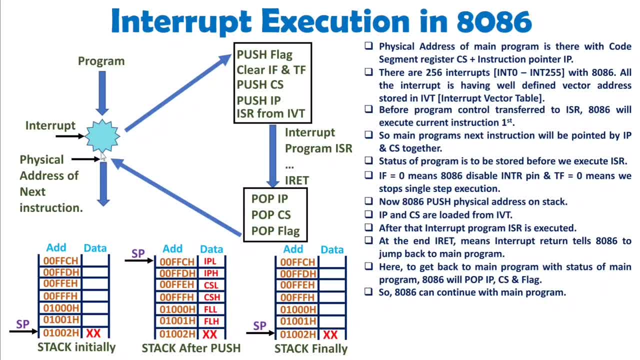 here, right. so with normal subroutine you will be having transfer of control from routine over here where you don't need to see what was the flag which was there over here, right. but in case of interp execution you will have to do push flag over here, right? so when you write, only return at that. 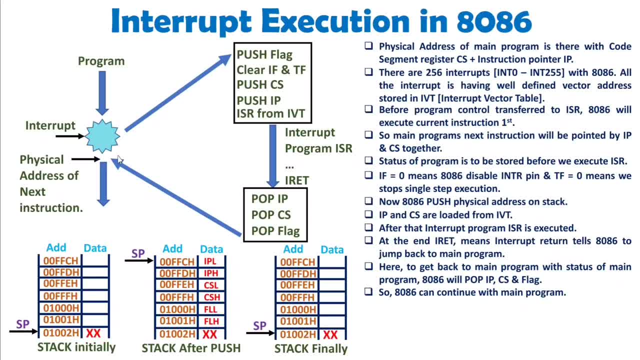 time you will have to retry status of program as well, right? that is one thing that you need to know. in terms of normal subroutine and interrupt subroutine, see, interrupt subroutine is subroutine, right, but that is bit different compared to normal subroutine. one more thing, my dear students, that you 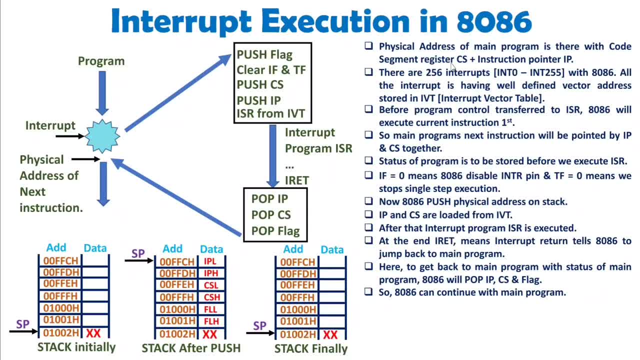 need to see here: with main program we have segment register and instruction pointer, right? so this main program is having segment register and instruction pointer, right? so this main program is having segment register and instruction pointer and this inter program that is also having segment register and instruction points, whatThere are students segment off the intervals program is different. 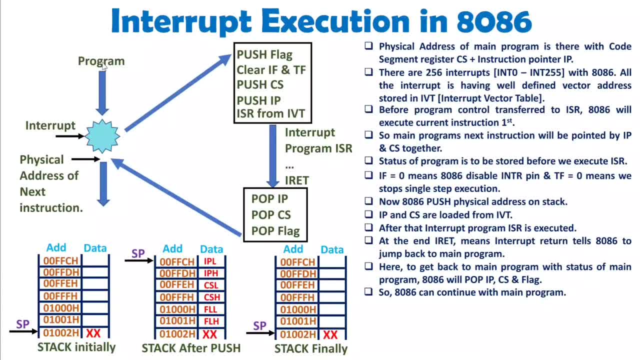 compared to main program. so what ever subroutine is happening with these interrupt execution, that will be intersegment subroutine. why the reason is: segment off this main program and segment of this inter program will be different, right? so inter in 8086 is inter segment branch or routine. that you can say why the reason is here. segment are different, right? so here it is.